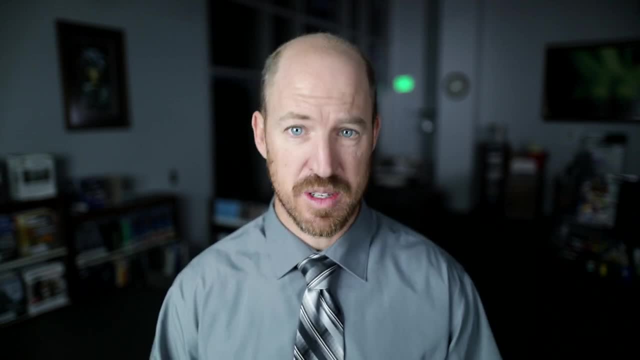 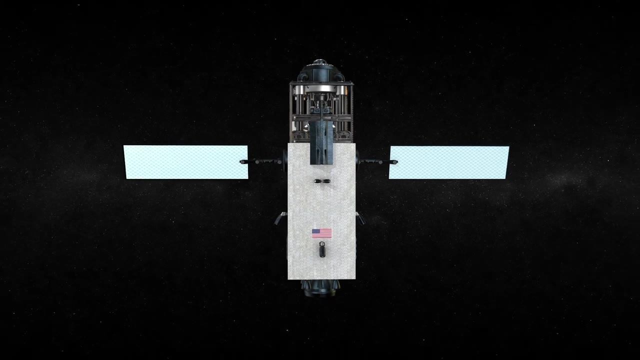 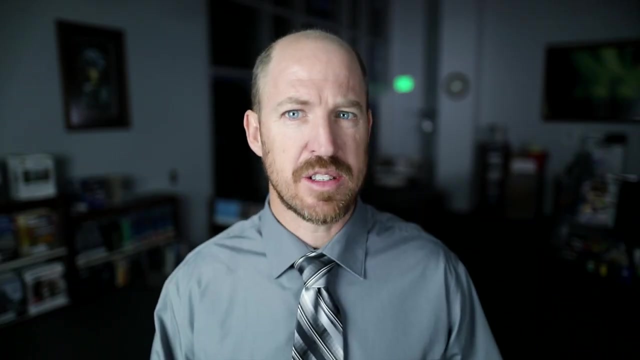 And the bus. It's all the parts that support the mission. Generally, the payload takes up approximately 30% of the total spacecraft mass budget and the rest of the subsystems or the bus is the remaining 70%. When designing spacecraft, we start with payload sizing. We determine the size, weight and power. 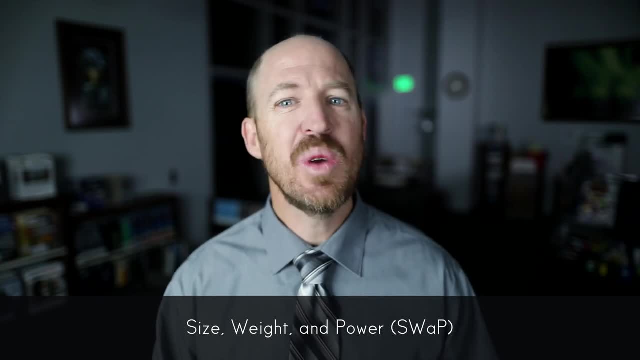 or swap requirements for the payload, Then we can estimate the swap for the spacecraft as a whole. This is the payload size. The payload size is the weight, weight and power. The payload size is the weight, weight and power or swap requirements for the payload. Then we can estimate the swap for the spacecraft as a whole. 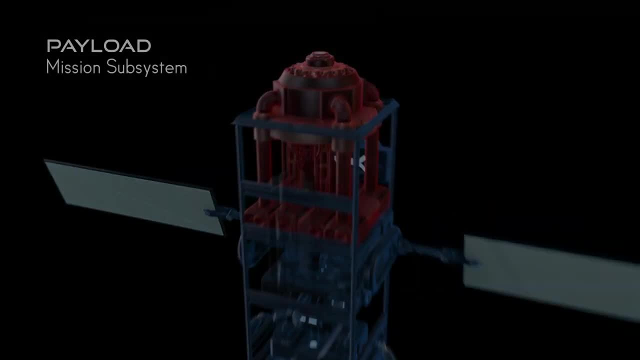 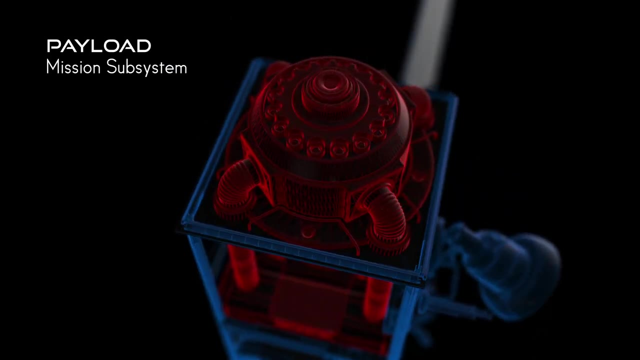 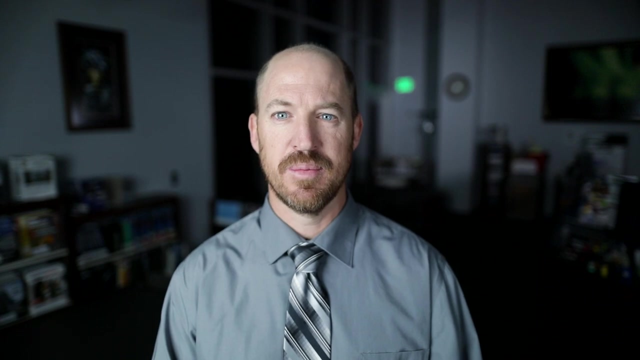 This process is very iterative, Starting with the payload or the mission. first we answer the question: why are we going into space? For examples of submission areas or payload types, please reference the electromagnetic spectrum series of educational aids. Once the payload is determined, we can move to all the supporting subsystems. 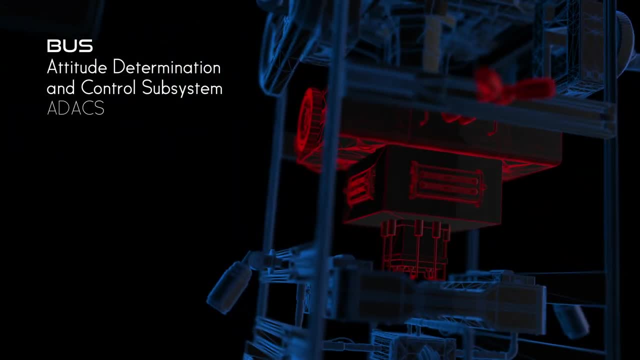 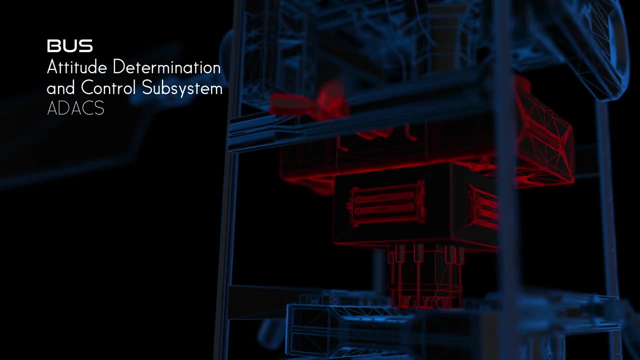 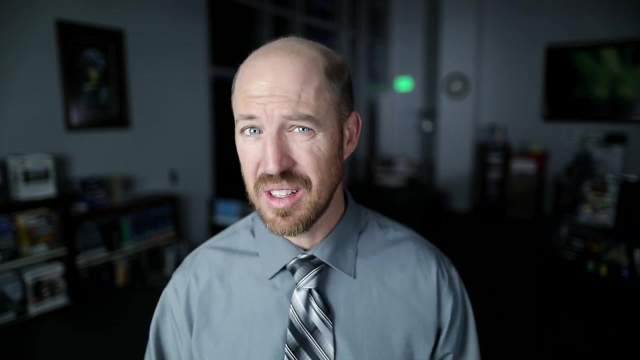 The first subsystem we are going to look at is the attitude determination and control subsystem, or simply referred to as 8X. The purpose of this subsystem is to control and monitor the rotation of the spacecraft. This subsystem answers the questions. where am I pointing? 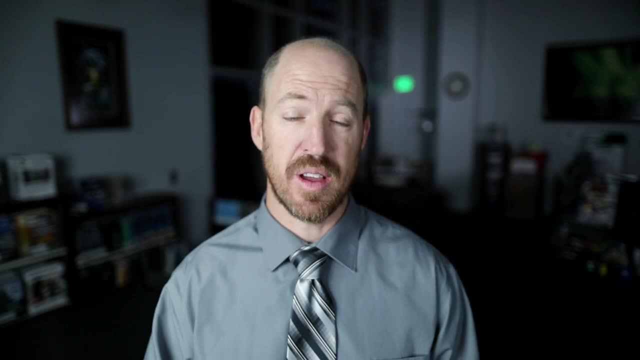 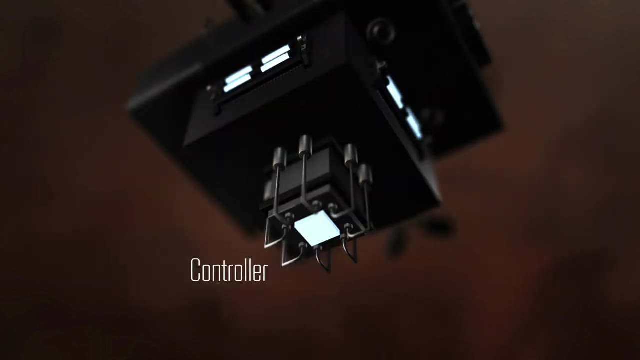 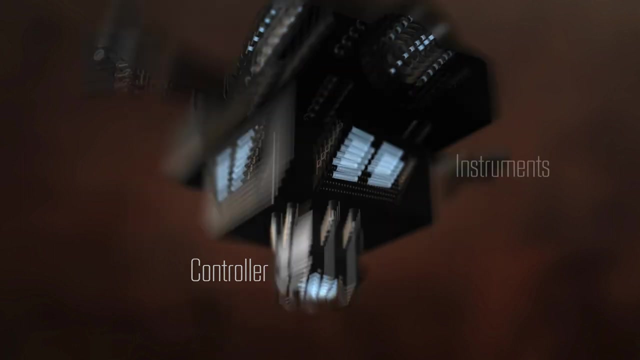 where do I want to point and how do I maneuver the spacecraft to point there? This subsystem is comprised of several components. The first major component is the controller or the computer that receives the commanded or programmed inputs for the desired direction to point. The next major components are the instruments that aim to control the spacecraft. 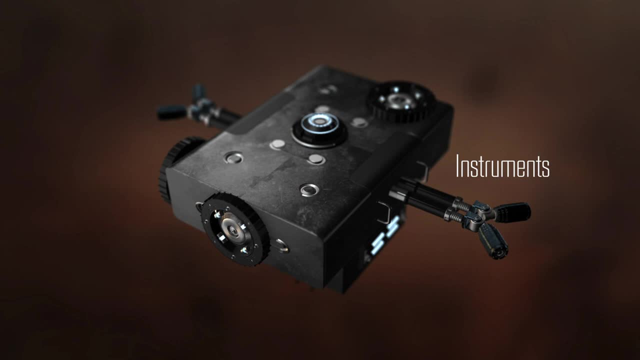 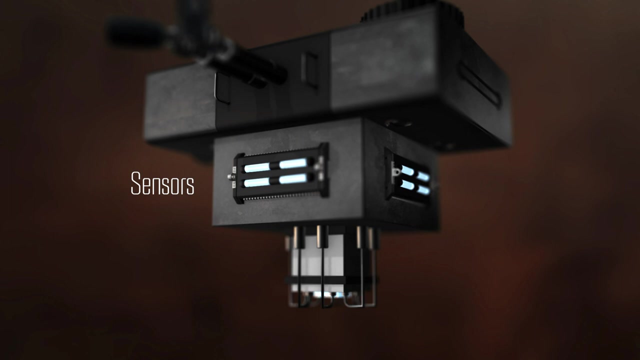 They can aid the spacecraft to move or rotate so it can point in the desired direction. Such instruments are reaction wheels, thrusters and magnetic torque. The last major component of this subsystem are the sensors. Sensors allow the satellite's orientation to be measured. 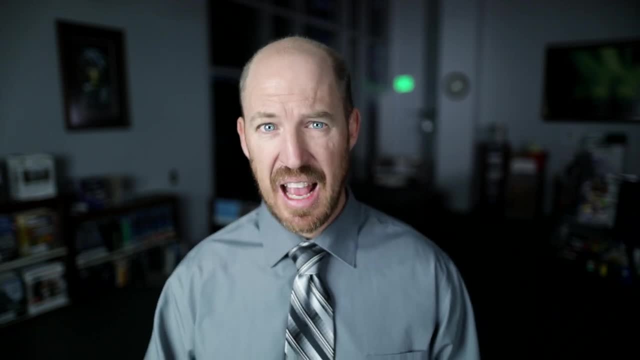 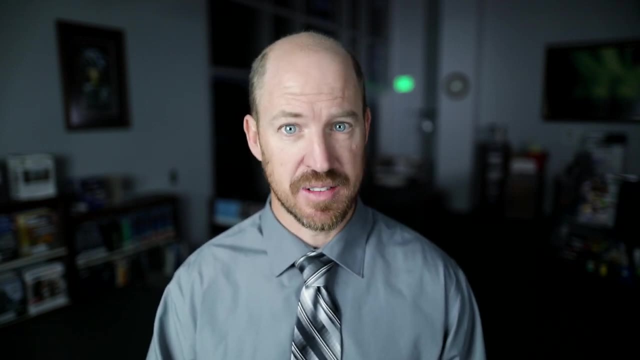 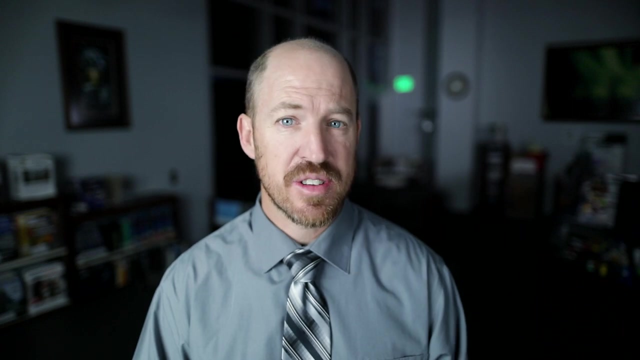 These sensors enable the satellite operator to determine the orientation of the satellite, answering the questions of where is it pointing, and eventually answers pointed in the desired direction. Examples of such sensors are Earth, Sun and Star sensors, gyroscopes and accelerometers and position navigation. 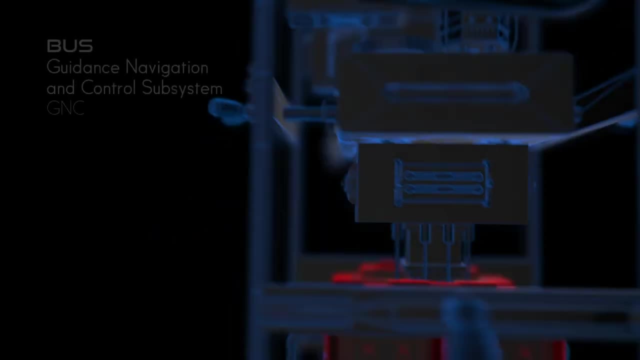 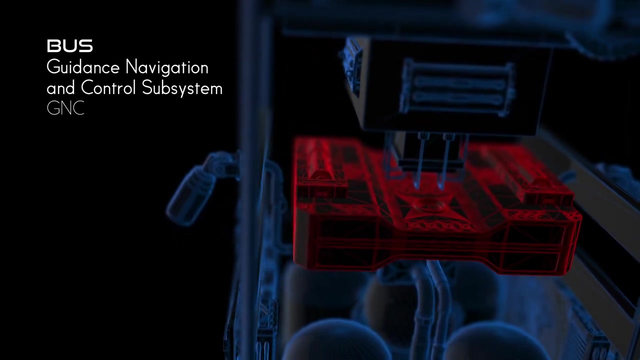 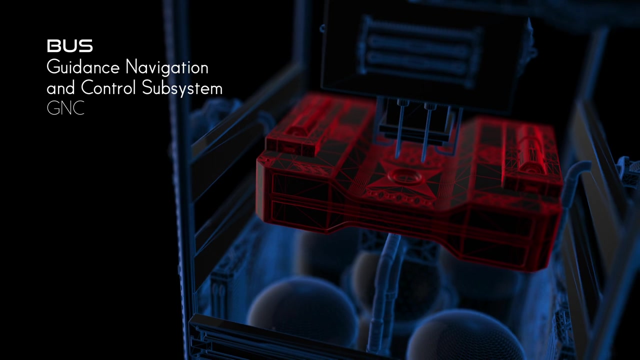 and timing, or PNT sensors. After ADACs, we move to the Guidance, Navigation and Control subsystem, or GNC. The purpose of the GNC is to control or maintain the orbit of the spacecraft and to move into a desired orbit. This answers the. 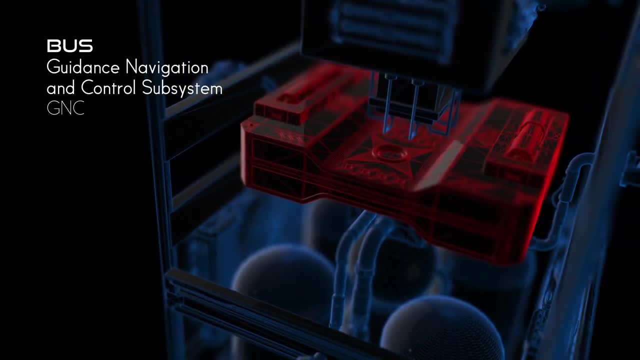 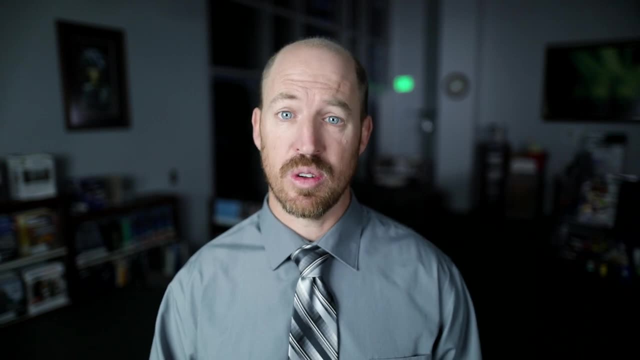 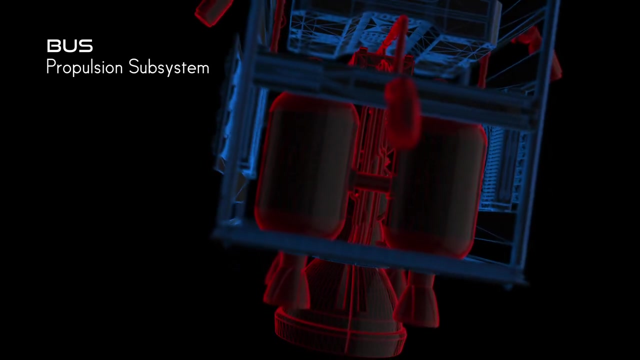 question: where is the spacecraft? The propulsion subsystem, which is described next, is the primary actuator for the Guidance, Navigation and Control subsystem. The propulsion subsystem aids the spacecraft to move into a desired orbit or maintains the satellite in its current orbit and performs station. 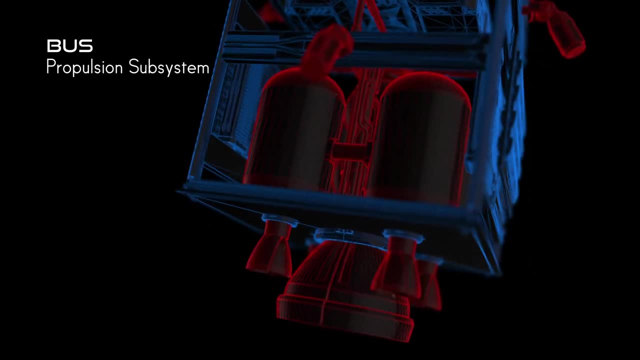 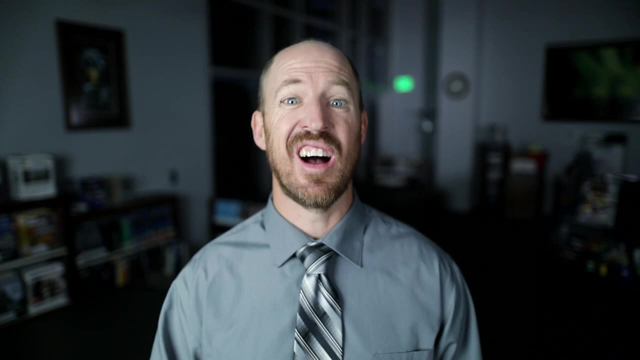 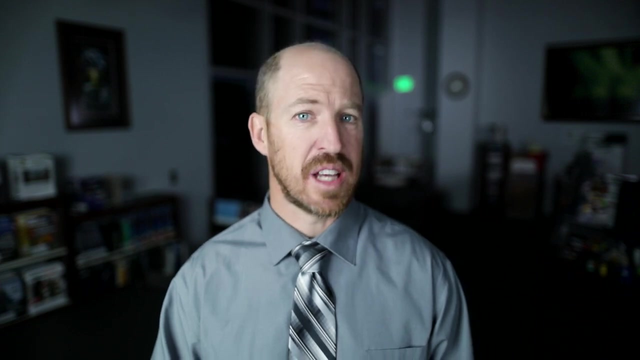 keeping operations such as firing a thruster to help maintain orbital altitude to overcome atmospheric drag. We will talk more on atmospheric drag and other environmental effects in the Space Environment Educational Aid. Many smaller satellites, such as nano or pico satellites, due to the complexity involved, do not have propulsion subsystems. 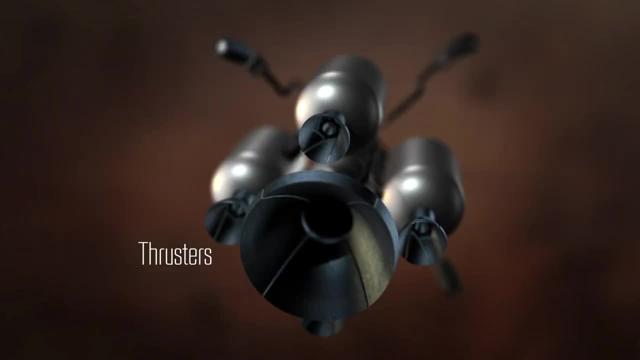 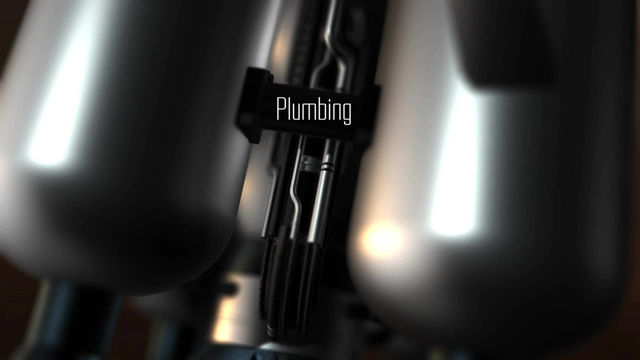 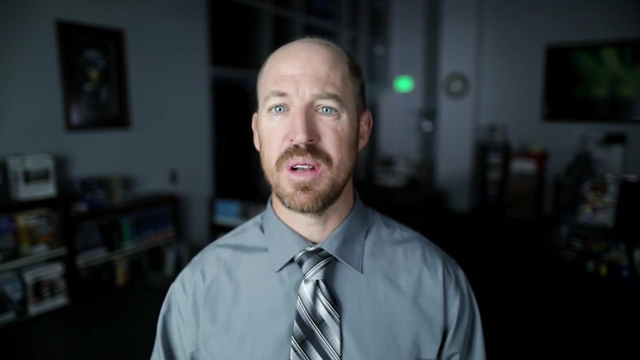 However, propulsion subsystems are made up by thrusters, propellant tanks and the plumbing which connects the tanks to the thrusters. We will discuss propulsion in greater detail in the Launch, Propulsion and Reentry Educational Aid, And for information on orbit types, please see the Orbit Types Educational Aid. 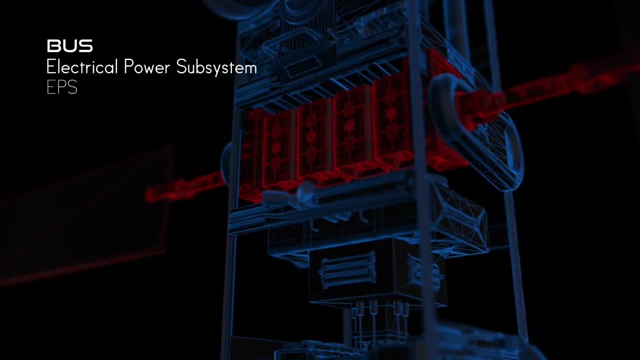 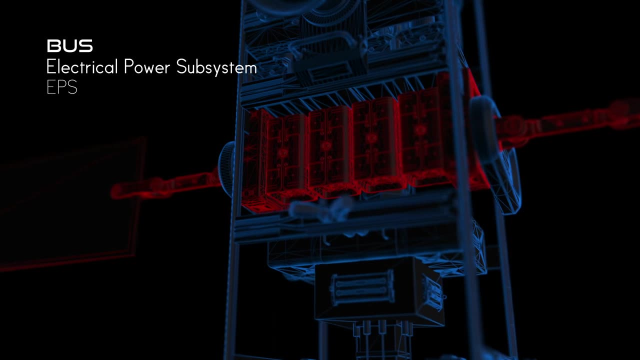 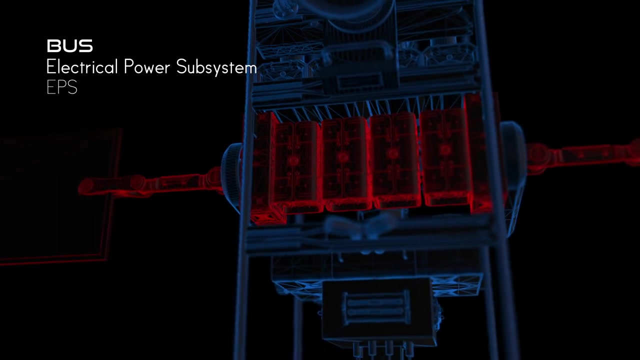 After propulsion we move to the electrical power subsystem, or EPS. The electrical power subsystem is responsible for the generation, storage and providing electrical power for the entire spacecraft. Most satellites use solar arrays to generate and provide electrical power to the spacecraft. Solar arrays are also providing power to the batteries for storage. 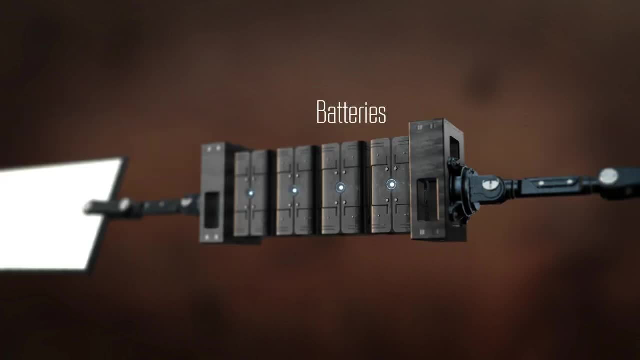 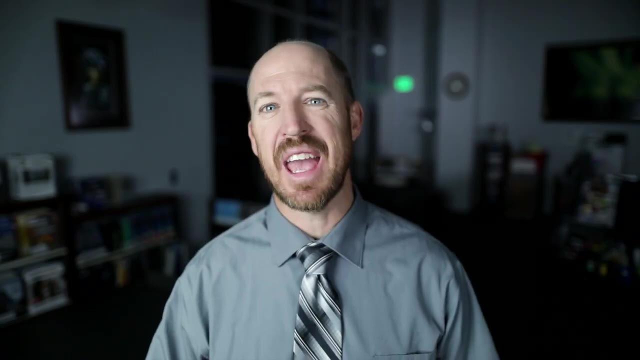 So, when the satellite is not in view of the sun, batteries are used to provide spacecraft power during this time of eclipse. Again, just as with ADACs, there is a computer, or, more specifically, a Power Management and Distribution, or PMAD, system. 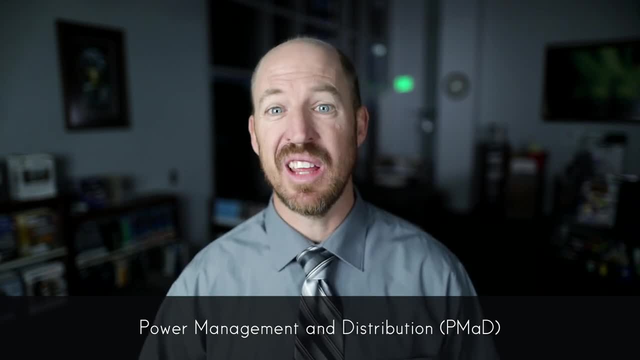 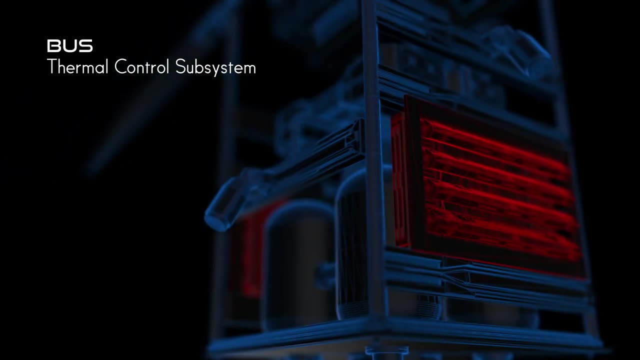 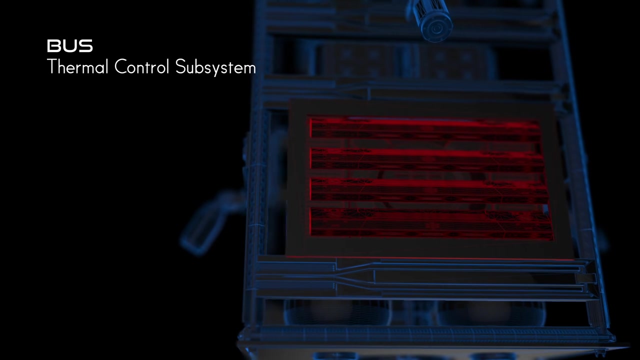 The PMAD is responsible for allocating power in the correct voltages and current to the rest of the satellite. The next subsystem is the Thermal Control subsystem. The purpose of this subsystem is to regulate and maintain the temperature throughout the spacecraft. The payload and all the other subsystems have temperature ranges which they optimally operate within. 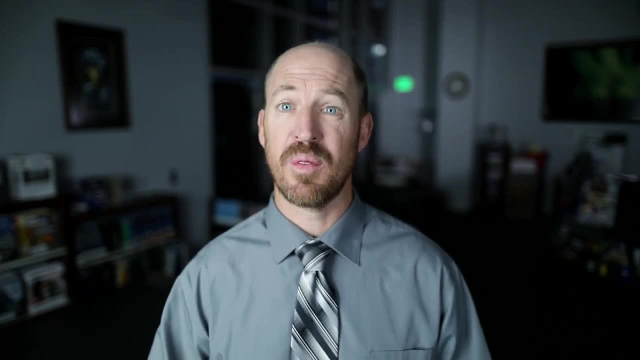 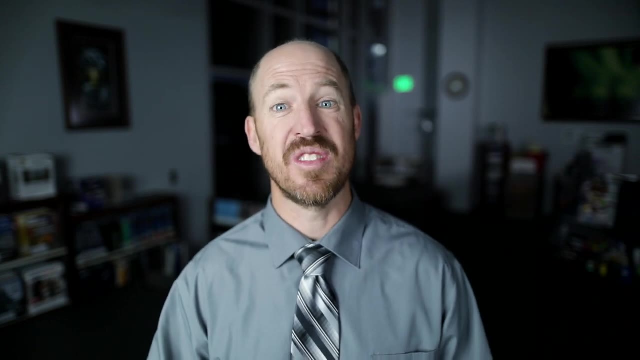 The typical source of heat that affects spacecraft come from the sun, Earth and internally from the spacecraft. The Thermal Control subsystem ensures temperature requirements of these subsystems are maintained. Primarily, it ensures that the temperature requirements of these subsystems are maintained. 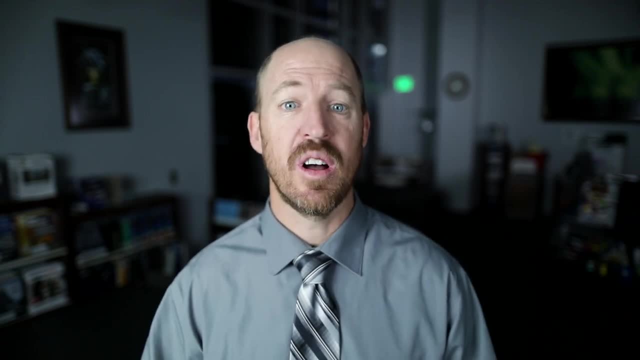 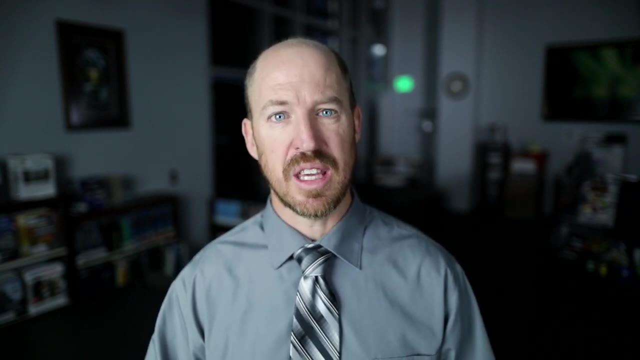 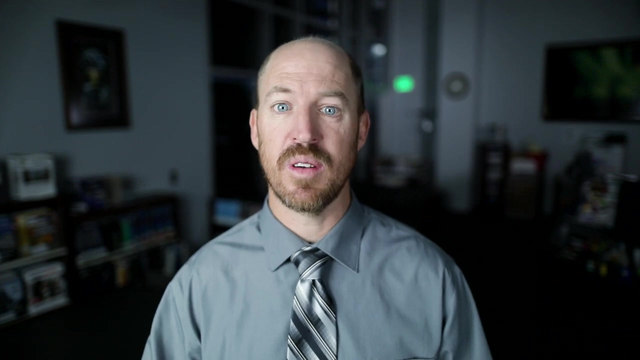 Insulation or protective coatings handle the majority of the thermal control needs of the spacecraft. Additionally, some other examples that spacecraft can use to manage thermal needs are radiators that emit heat or louvers, which can be opened and closed like Venetian blinds to expose or cover the radiators. 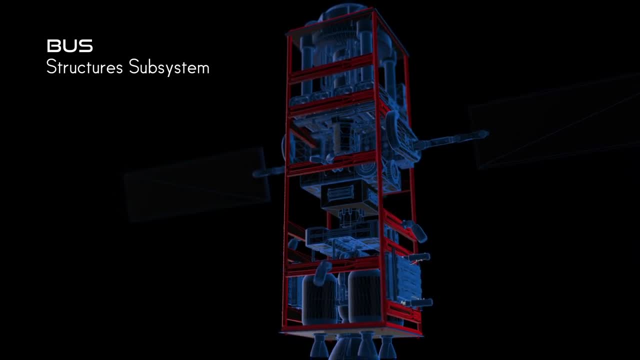 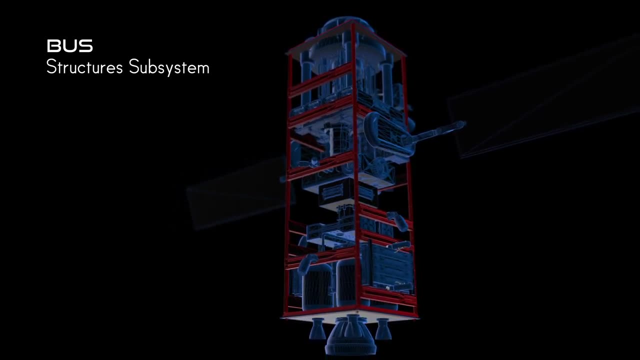 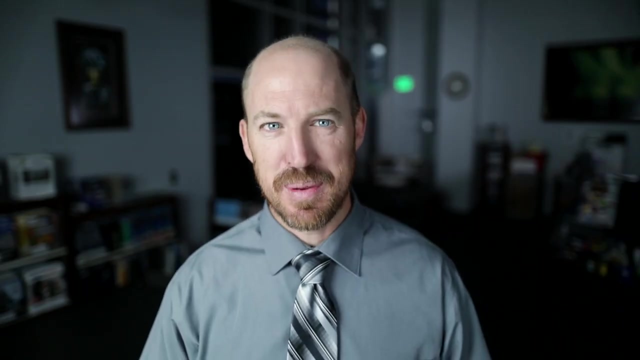 The next subsystem is structures. Think of structures as the frame or chassis of an automobile. Everything is attached to it. So with a spacecraft, every subsystem is attached to this subsystem, payload included. The size of the structure is dependent upon the payload, its requirements and the launch vehicle the satellite will ride to get into orbit. 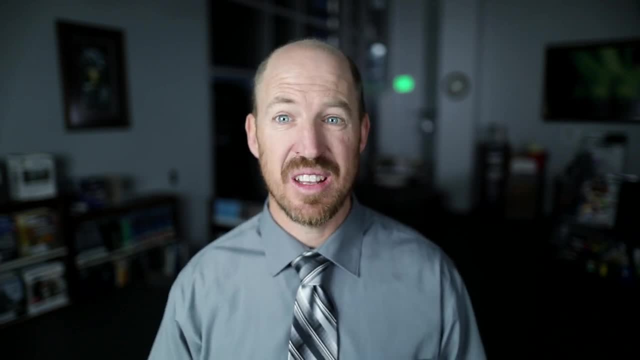 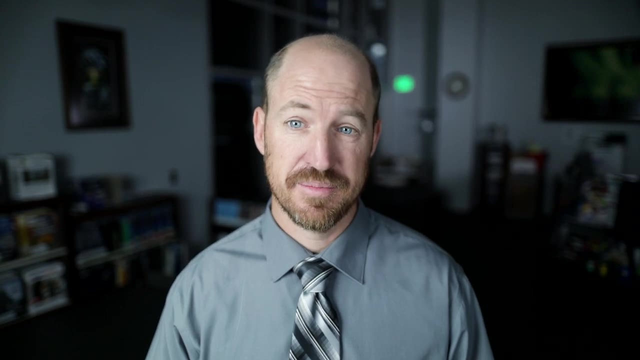 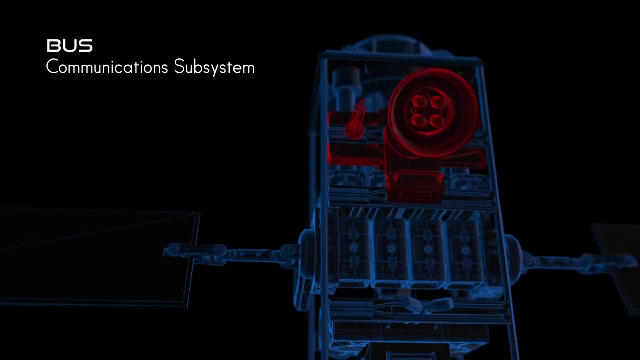 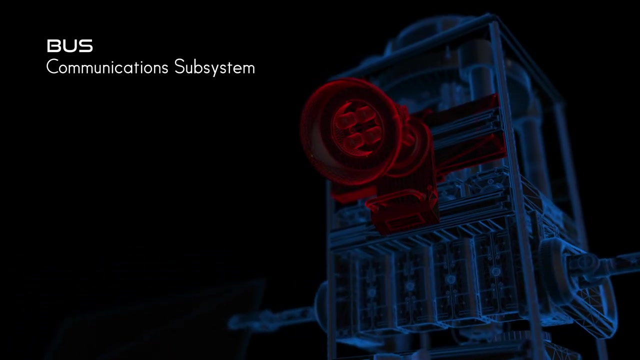 Structure sizes can range from the size of a soda can to the size of a large bus. Many satellite manufacturers have a standard structure for varying mission needs. The next subsystem is the Communications subsystem. This subsystem allows the ground to send commands to the satellite and disseminate information such as satellite position and payload data to the ground. 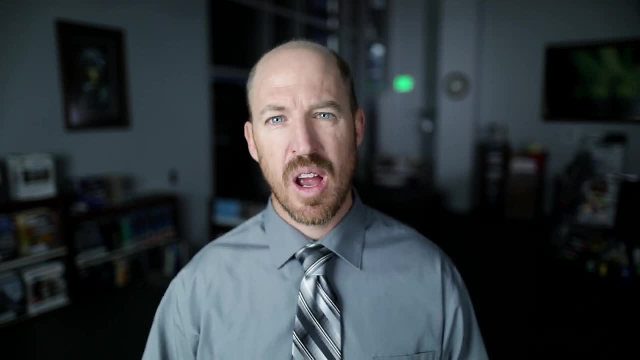 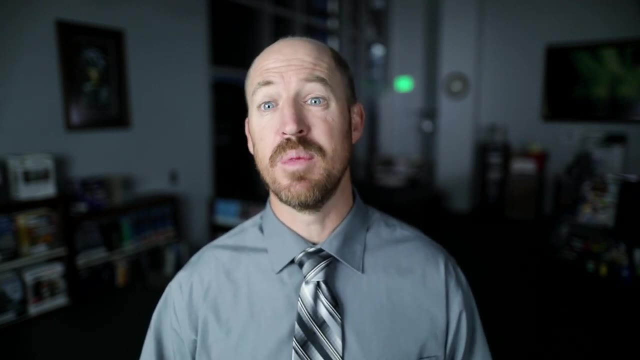 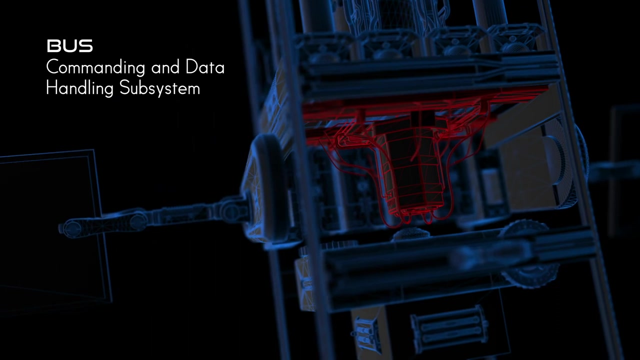 This subsystem is primarily made up of transmitters, receivers and antennas. It is important to note that communications can be the mission of the spacecraft, but most spacecraft have a need to receive commands and send telemetry. The last subsystem we will cover is the Commanding and Data Handling subsystem. 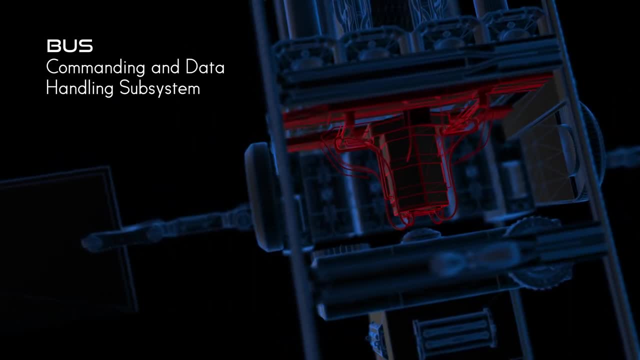 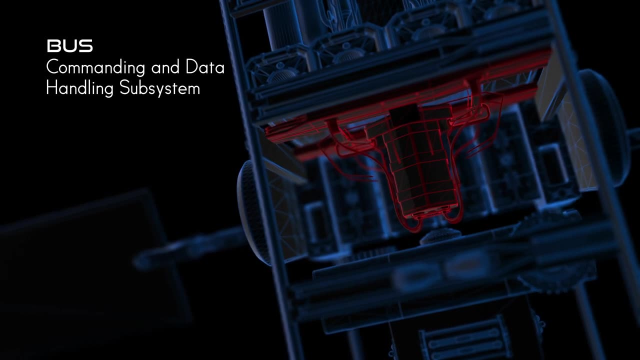 The last subsystem we will cover is the Commanding and Data Handling subsystem. The last subsystem we will cover is the Commanding and Data Handling subsystem. This subsystem is the brains of the spacecraft. It manages, stores and controls all ground commands, payload data and telemetry during all phases of the spacecraft mission. 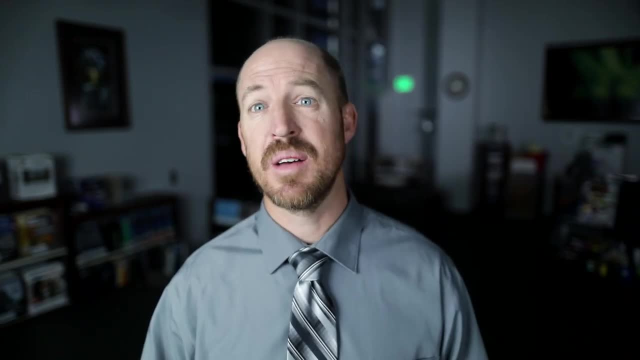 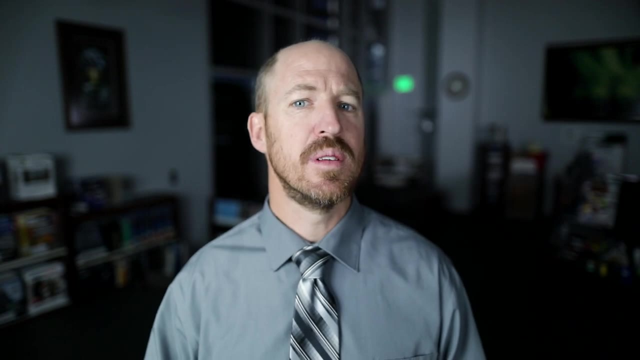 To do all this commanding and data handling. this subsystem is comprised of several elements. The first element is the CPU. It works like a typical computer but is hardened to operate in a space environment. The next element is the CPU. It works like a typical computer, but is hardened to operate in a space environment.